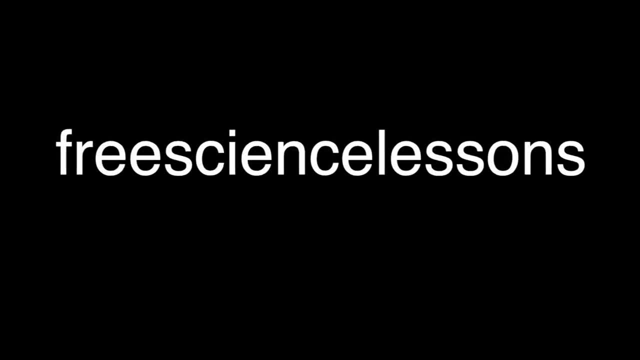 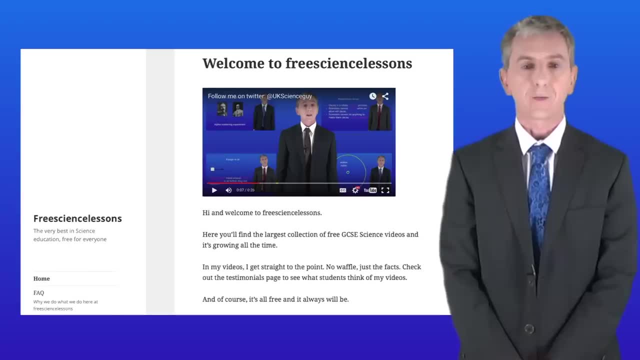 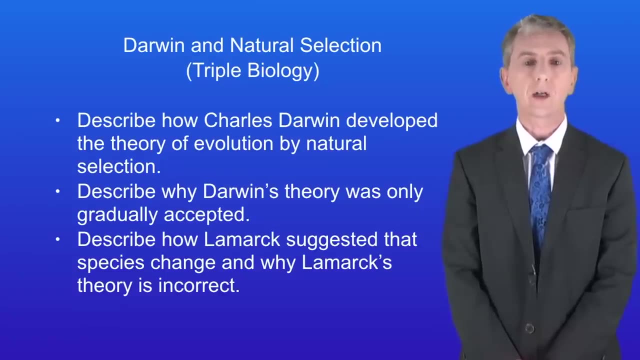 Hi and welcome back to freesciencelessonscouk. By the end of this video, you should be able to describe how Charles Darwin developed the theory of evolution by natural selection. You should then be able to describe why Darwin's theory was only gradually accepted And finally, 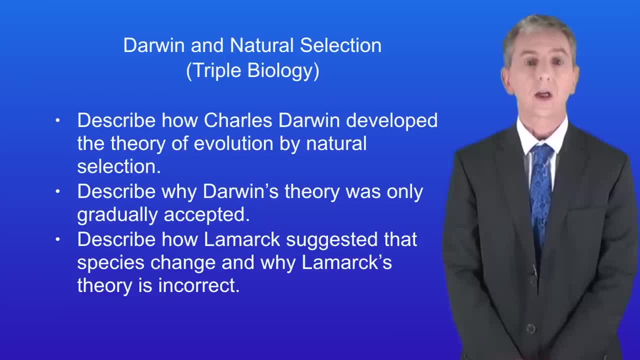 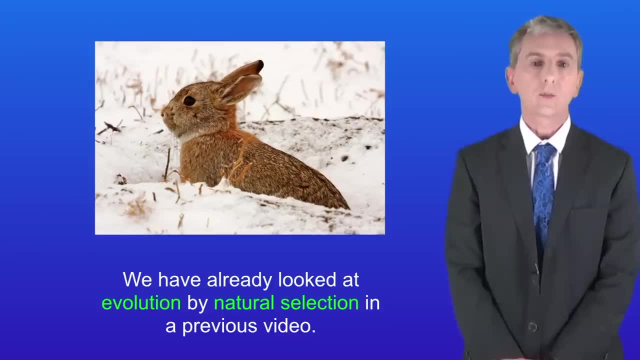 you should be able to describe how Lamarck suggested that species change and why Lamarck's theory is incorrect. And all of this is for triple biology students only Now. we've already looked at evolution by natural selection. in a previous video We looked at 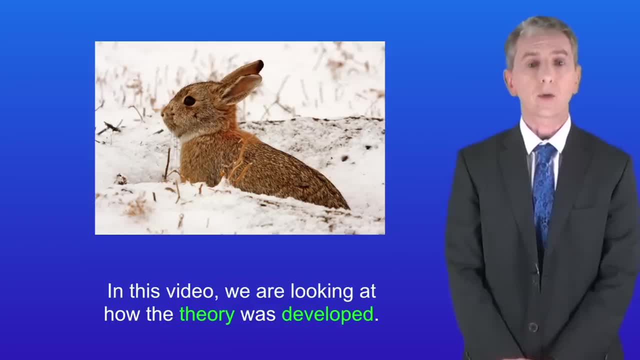 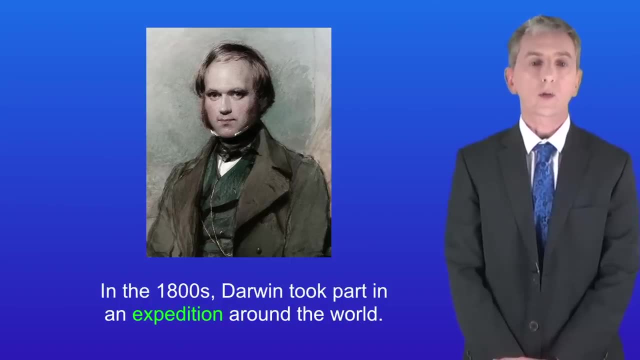 the example of rabbits. In this video we're looking at how the theory was developed. I'm showing you here a picture of the scientist Charles Darwin. In the 1800s, Darwin took part in an expedition around the world and he collected a vast number of different animals. 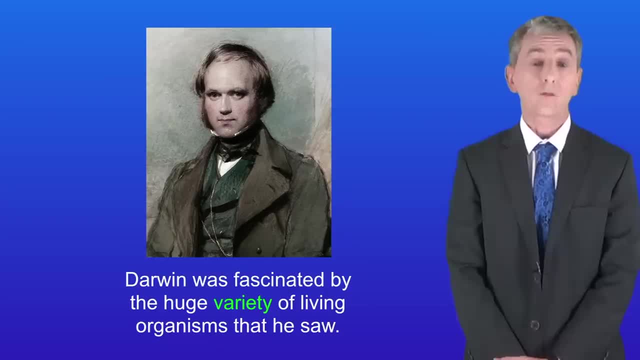 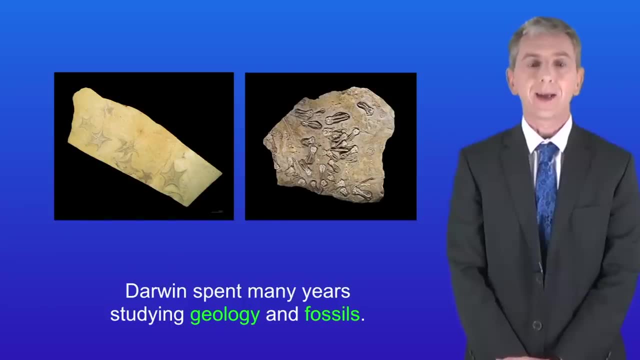 and plants. Darwin was fascinated by the huge variety of living organisms that he saw. He began to wonder how all of this variety developed. Darwin spent many years studying geology and fossils. These fossils showed that many species of animals and plants alive today are similar to extinct species. After many years of experimentation and discussion, Darwin 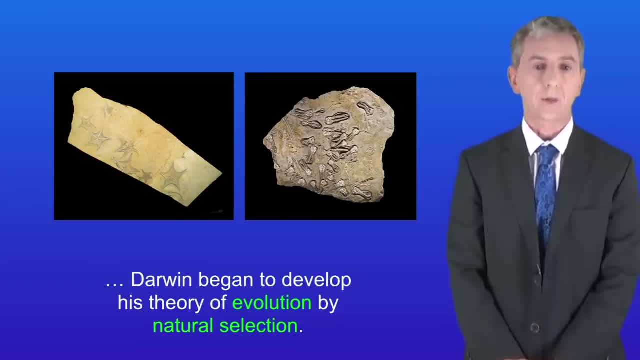 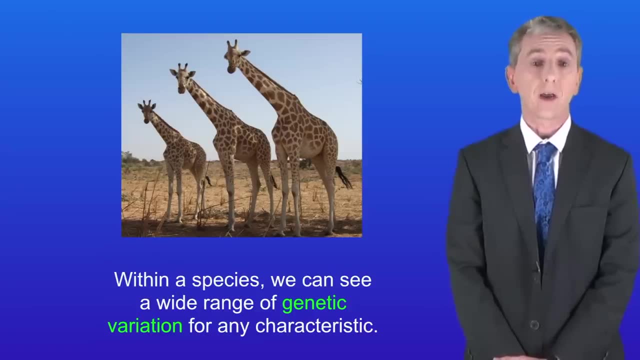 began to develop his theory of evolution by natural selection. And again, it's really important that you learn this. Firstly, within a species we can see a wide range of genetic variation characteristics. For example, if we look at giraffes, we can see that some giraffes 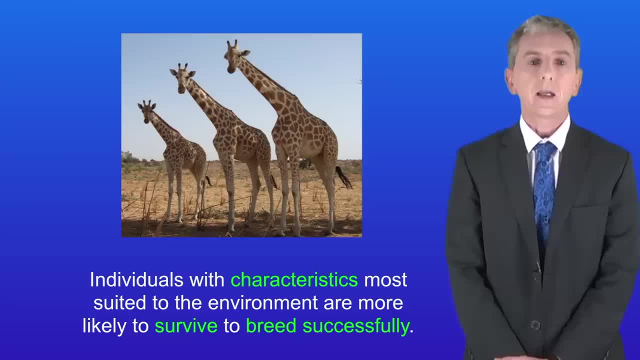 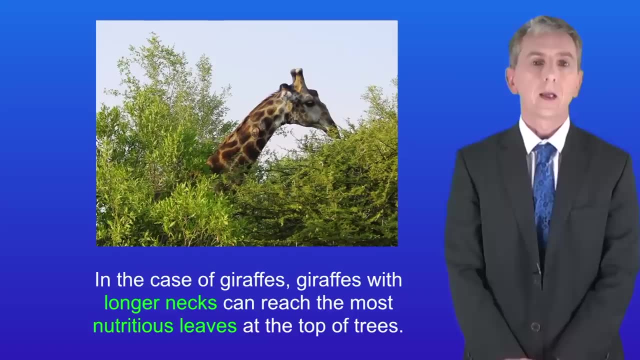 have got longer necks than others. Secondly, individuals with characteristics most suited to the environment are more likely to survive, to breed successfully. In the case of giraffes, giraffes with longer necks can reach the most nutritious leaves at the top of trees. These 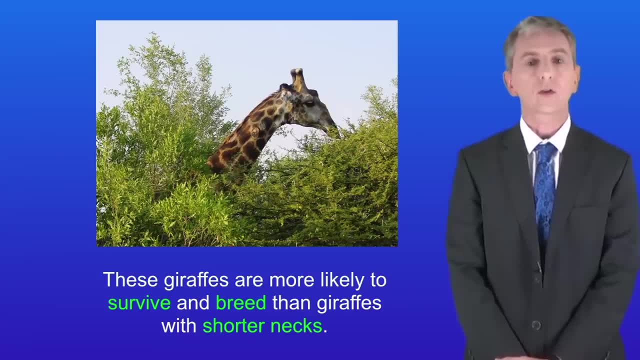 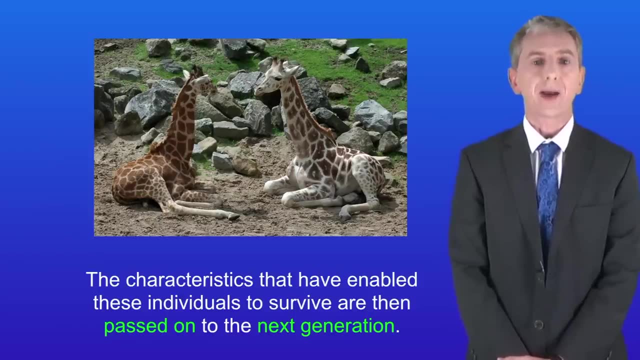 giraffes are more likely to survive and breed than giraffes with shorter necks And, lastly, the characteristics that have enabled Darwin to develop his theory of evolution have been developed to enable these individuals to survive, or then passed on to the next generation. 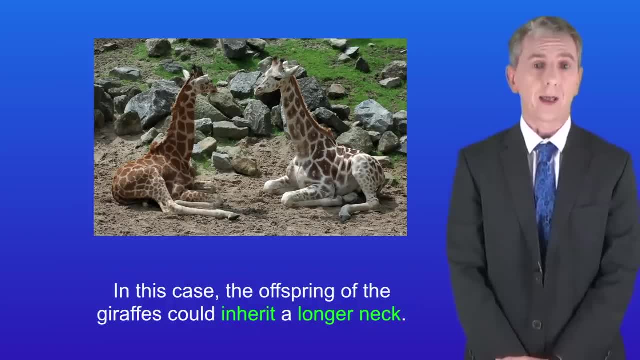 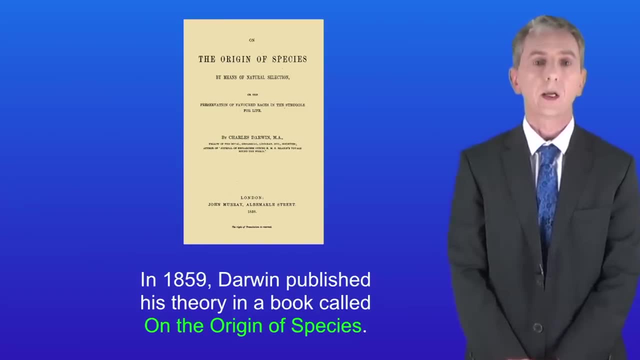 So in this case, the offspring of the giraffes could inherit a longer neck. Now, in 1859, Darwin published his theory in a book called On the Origin of Species. Darwin's theory was extremely controversial and was only gradually accepted. You need to be able to explain why At the